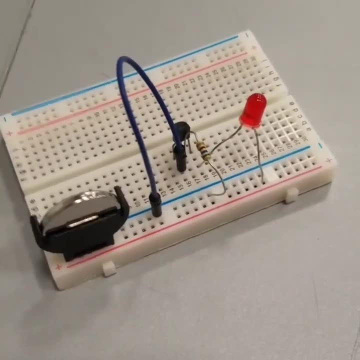 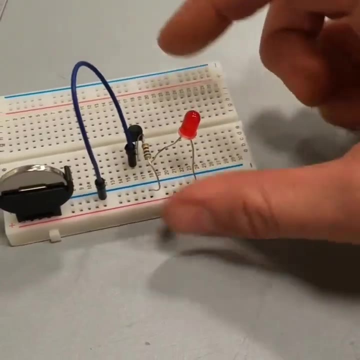 Okay, so here's a quick overview on transistors, because they can be kind of complicated to figure out what they're actually doing. So this is an NPN transistor, which means that the right pin is the collector which is connected to the LED. 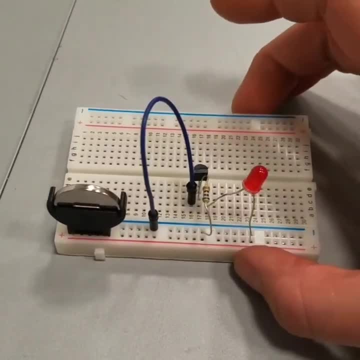 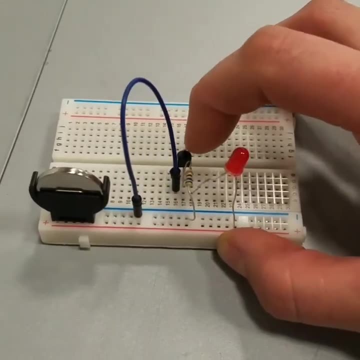 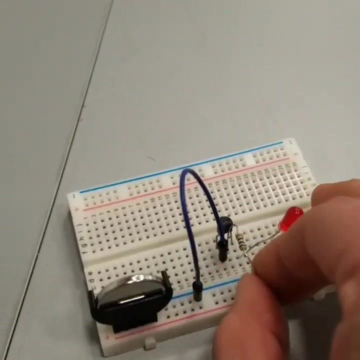 The middle pin, per usual, is the base that's connected to the resistor, and the left pin is the emitter. So when there is no voltage on the base pin, no current is allowed to flow between the collector and the emitter. But when there is a voltage on the middle pin- which let me see if I can do this with one hand- 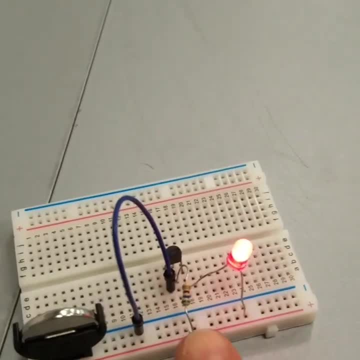 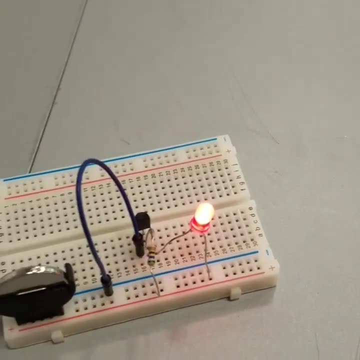 Haha, boom, There we go. So now there is a voltage on the base pin through the resistor, which means that it allows current to flow from the collector to the emitter and it completes the circuit. So this is an example of how transistors can act as a switch. 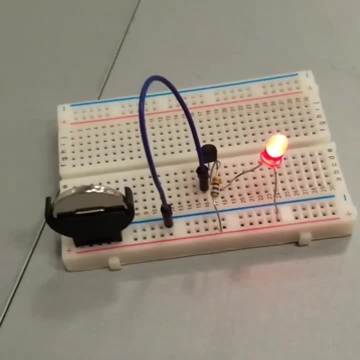 Yay, transistors, Woohoo, Alright, so let me know if you have any questions, and you should totally try and make this circuit on your own. Woohoo, Thanks for watching.